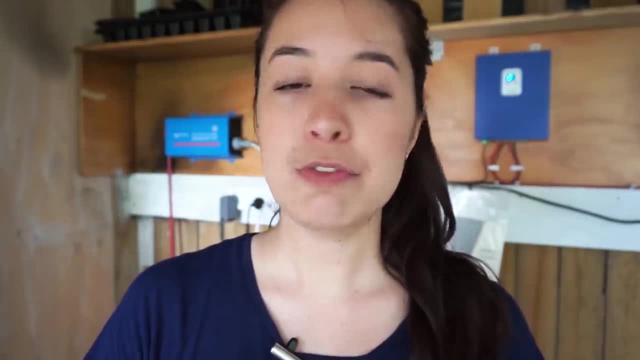 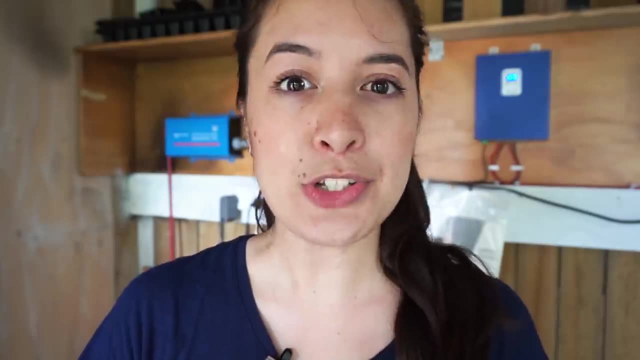 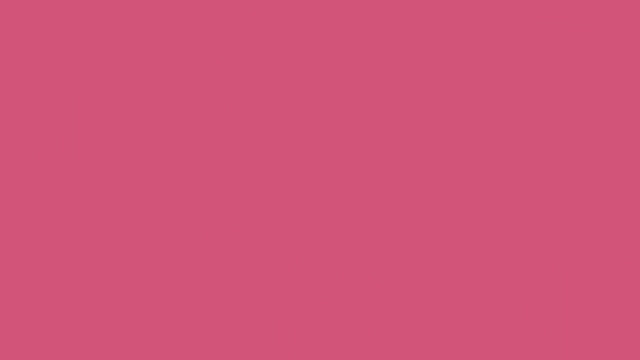 computer science accidentally created, but it was created from trying to answer a very abstract question about the foundations of mathematics. This story highlights an incredible turn of events, a brilliant thinker and the interconnectedness of two fields. The story starts with an extraordinary man named David Hilbert. He lived at a very exciting time in the history of mathematics. See. 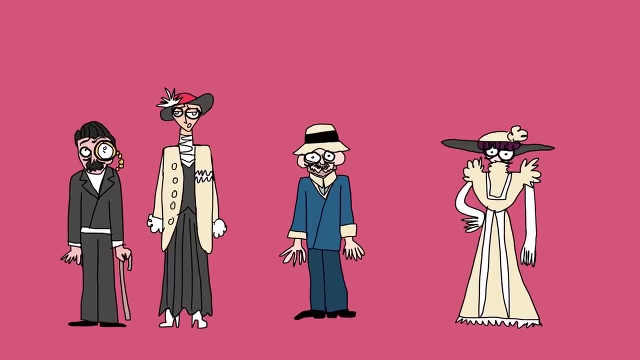 back in the day he was a computer scientist. He was a computer scientist. He was a computer scientist. See, back in the day he was a computer scientist. He was a computer scientist. He was a computer scientist. In the 1900s it had come to light that no one was really sure what they were studying when they 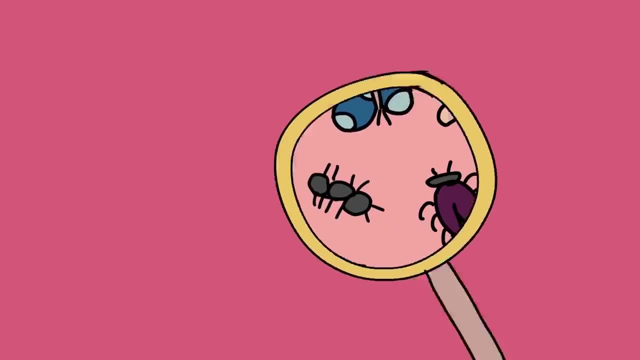 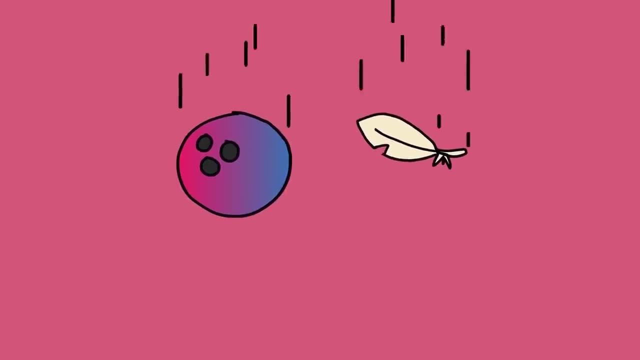 were studying mathematics. When we study biology, we're studying living things that exist in the real world. When we study physics, we're studying real world phenomena which we can verify via experiment. But math, Was it the study of real world objects or abstract entities? 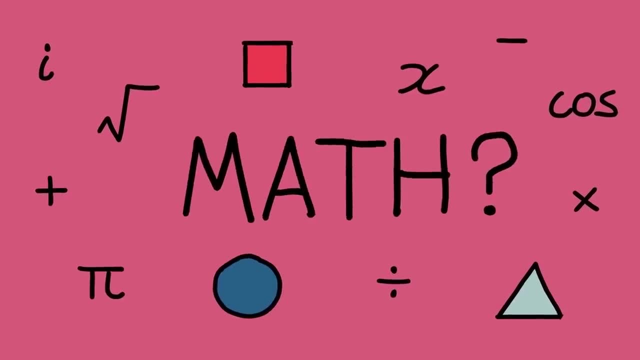 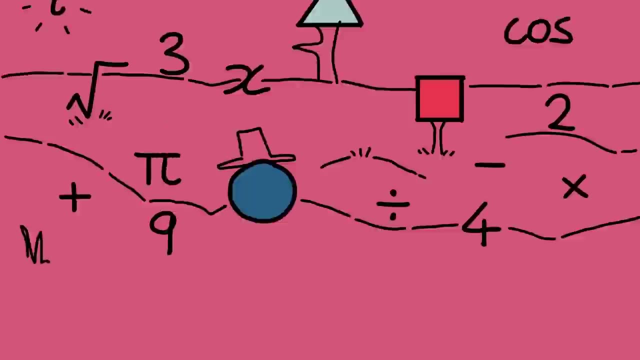 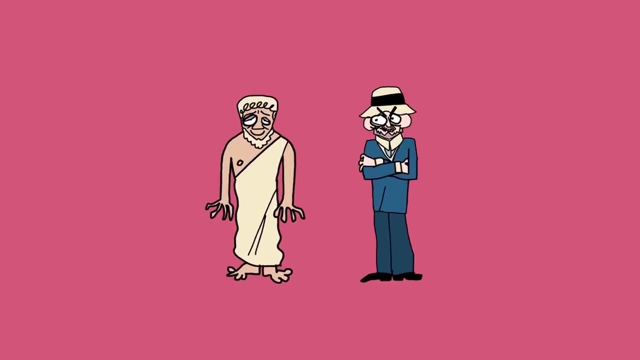 Did it exist in our minds or in some other realm of existence? The ancient Greek philosopher Plato thought that mathematical objects, shapes, numbers and the relationships between them belonged to their own ideal world, separate from ours. He called it the world of forms. But Hilbert wasn't a fan, He was a modern day man. 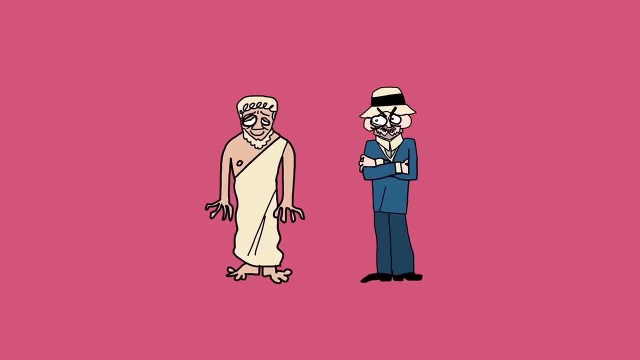 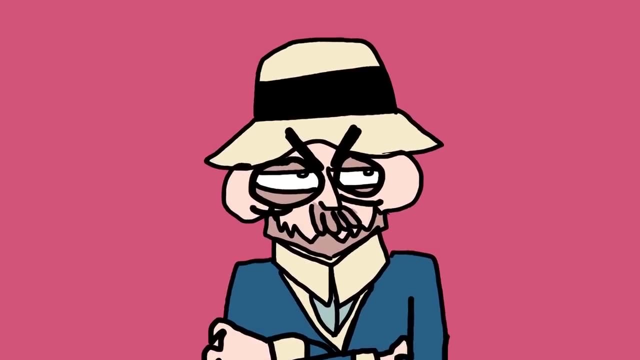 and the Platonist view was too mystical and airy-fairy for his liking. An idealized world of forms, Please. Hilbert was interested in down-to-earth matters, what could and couldn't be proven? Another prevailing view put forward by the German philosopher Immanuel Kant. 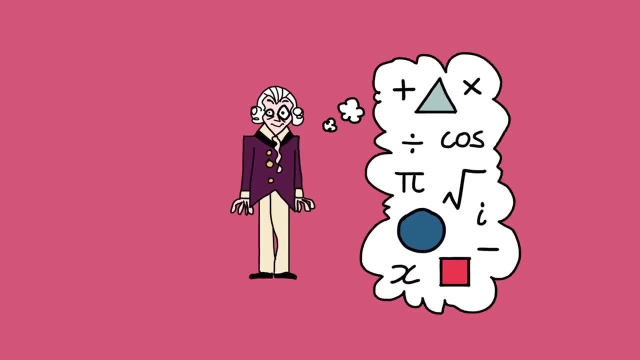 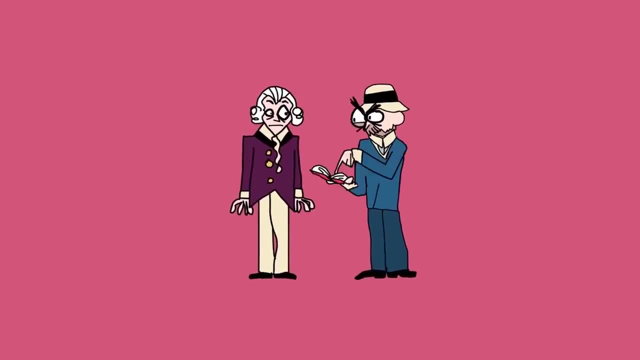 was that math was a mental construct based on our intuition. But Hilbert had a problem with this too. After all, intuitions could often lead us astray. The fact that the word paradox exists in the English language is evidence of that. 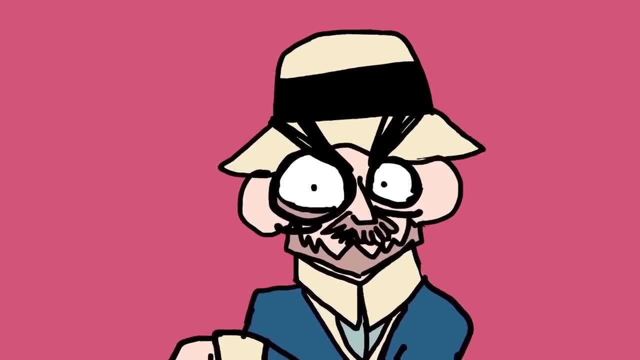 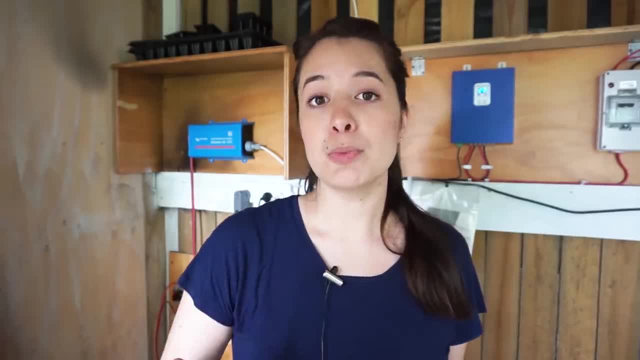 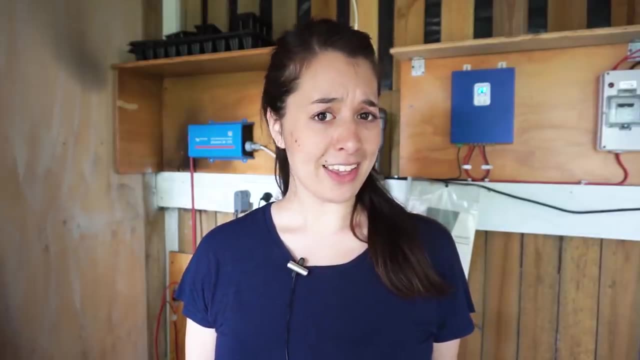 These differing viewpoints greatly irritated Hilbert. It's not uncommon to have multiple viewpoints in other disciplines. Literature, for example, is praised for being able to have multiple interpretations of the same thing. Even physical laws are revised and changed over time, But math. 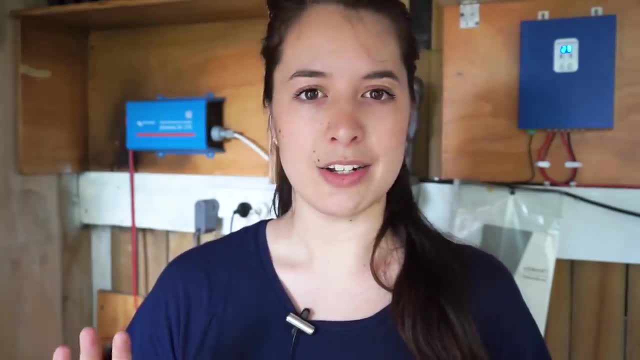 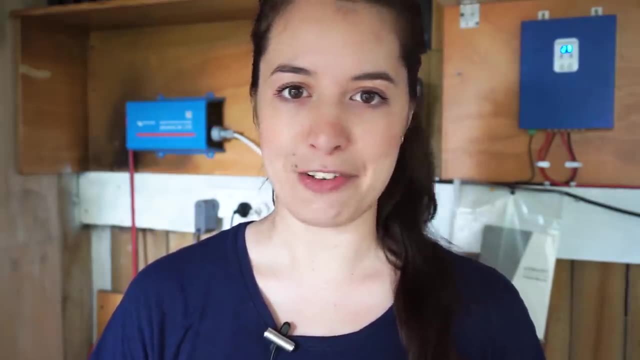 Oh no, This just wouldn't do. Math was regarded as different from the other disciplines. the epitome of certainty, The fact that 2 plus 2 equals 4, would never be revised and changed, And it just wasn't good enough that different mathematicians had different interpretations. 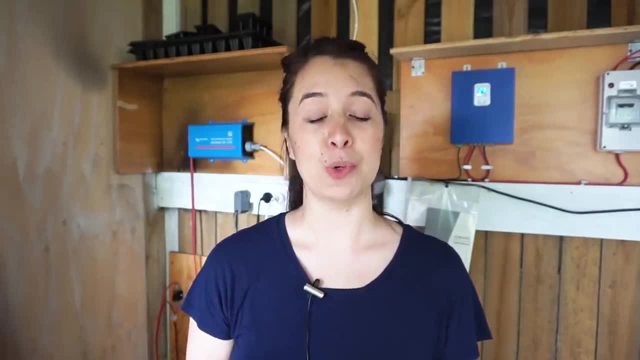 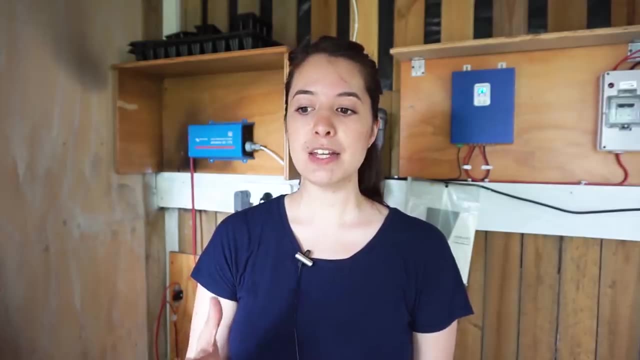 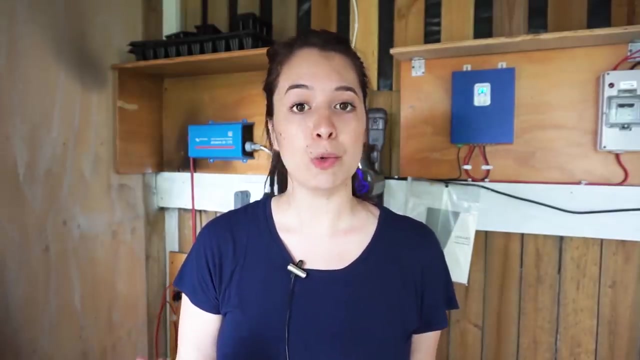 about what it meant. Aside from the prestige of math being called into question, these differing opinions had practical problems too. Those who agreed with Kant's intuitionism didn't believe that the idea of infinity fit within mathematics. Those who thought that logic was the foundation of math ran into logical paradoxes and inconsistencies. 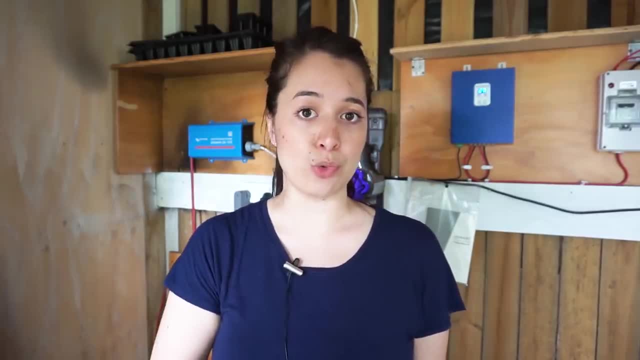 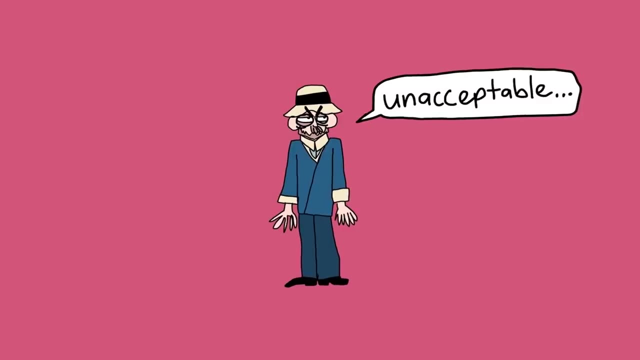 that limited what they could and couldn't do in comparison with the other schools of thought. You couldn't have different mathematicians playing by different rules. This was just unacceptable, and Hilbert was going to do something about it. He proposed a crazily ambitious program to axiomatize all of mathematics. 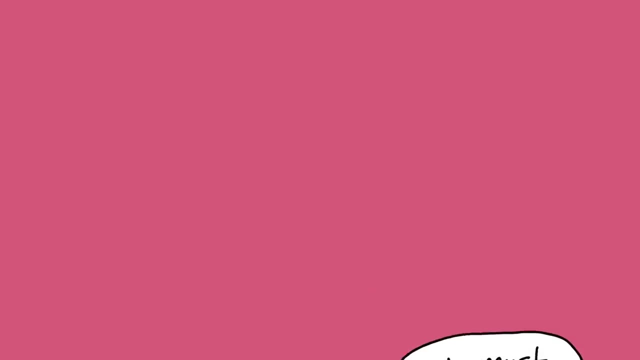 This sentence requires some explaining, See, Hilbert thought that if we treat math as nothing more than a formal system, there could be no more disagreements about what was and wasn't allowed. So what is a formal system? Well, it's an alphabet or a set of meaningless symbols which can be manipulated according to. 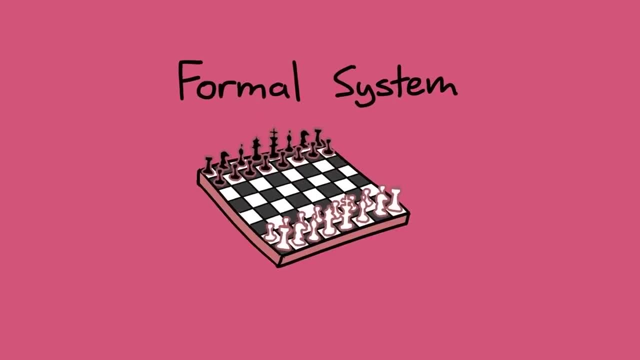 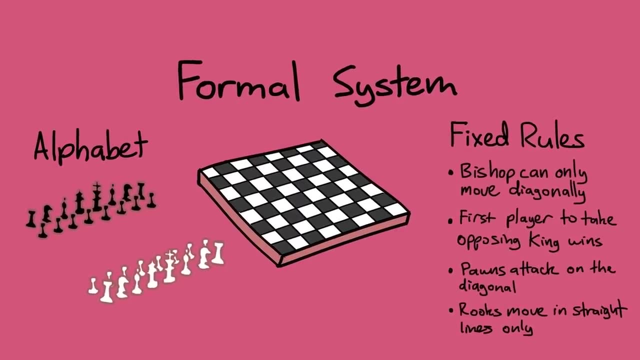 a fixed set of rules. Chess is a formal system. The alphabet are the pieces which are manipulated according to a fixed set of rules. It's important to note that the pieces and the rules don't have any meaning outside of the game. Hilbert thought that this was how we should view mathematics. 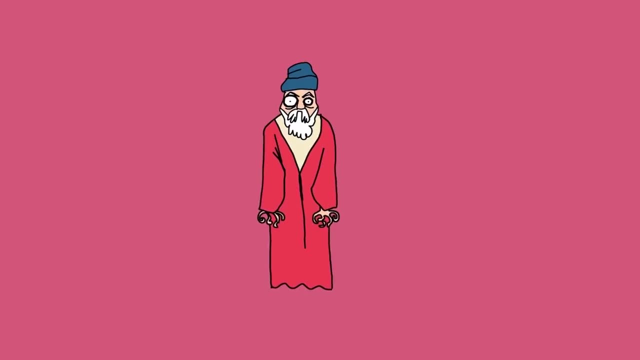 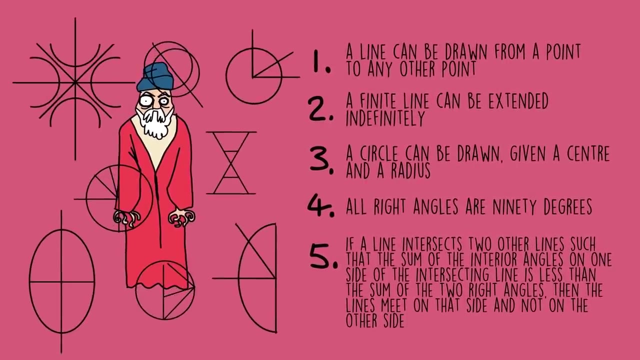 Something similar had been done by Euclid, on a much smaller scale. The whole system of Euclidean geometry was born by putting forward five self-evident axioms and the rules of how to build upon them. Equipped with these axioms, we don't need to know whether a triangle lives in the 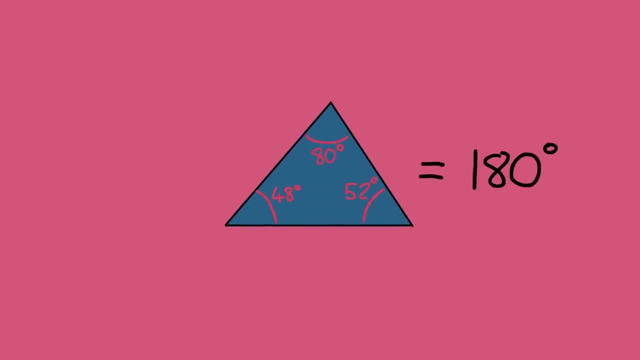 world of forms or in our heads, to know that its angles always add to 180 degrees. So in this way Euclidean geometry can be seen as a formal system. Hilbert wanted to do something similar: to find the foundational axioms for a formal system for. 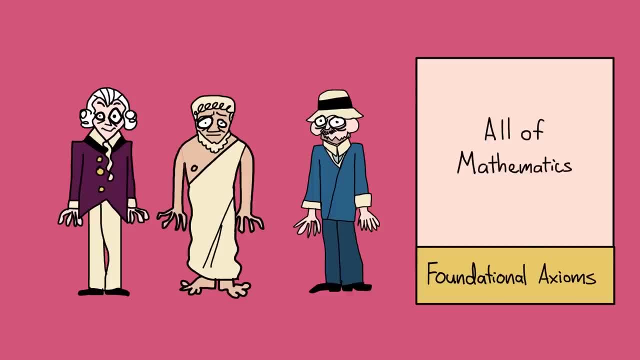 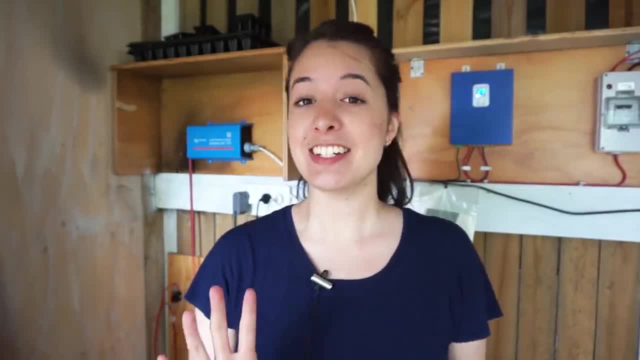 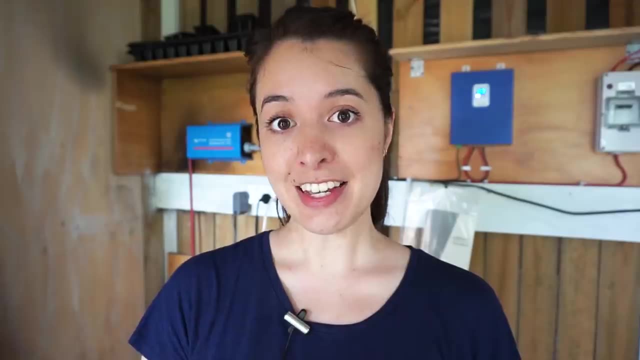 which all of mathematics could be built upon. This would eliminate any disagreements about what was and wasn't allowed. This was a monumental task and, to start, Hilbert thought about the three main things you would want in a foundational system of mathematics: Consistency, completeness. 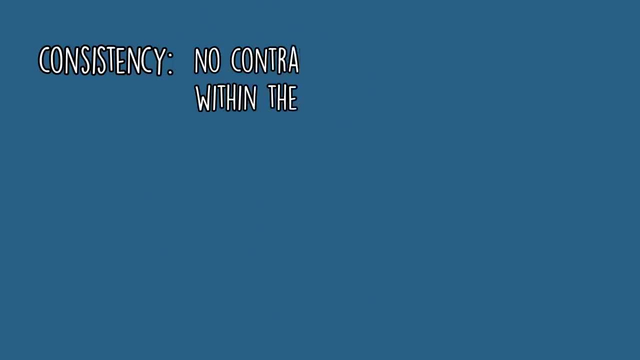 and decidability. Consistency means that no contradictions can be proven within the system. For example, you can't prove that 2 plus 2 equals 4 and that 2 plus 2 doesn't equal 4.. Inconsistencies would render the entire system. 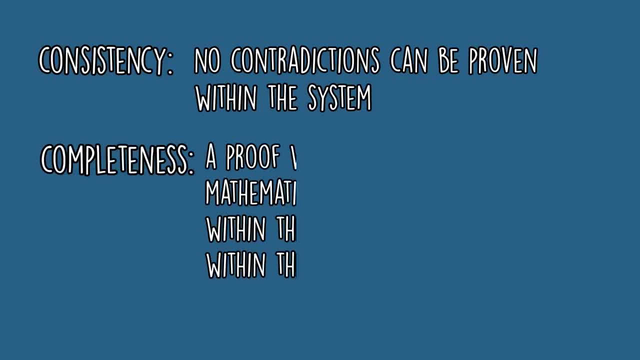 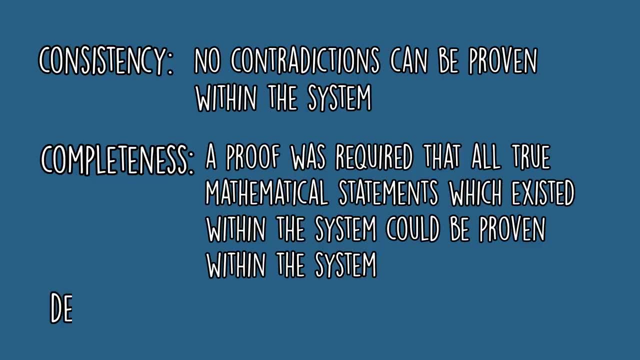 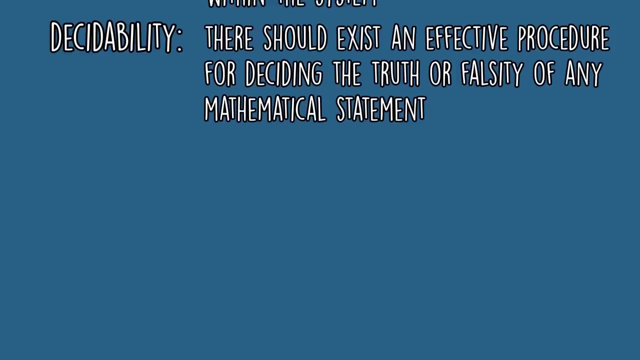 useless. Completeness means that a proof was required that all true mathematical statements which existed in the system could be proven within the system. And finally, decidability: This was the idea that there should exist an effective procedure for deciding the truth or falsity of any mathematical statement. For example, if, given the statement, P plus Q equals Z. 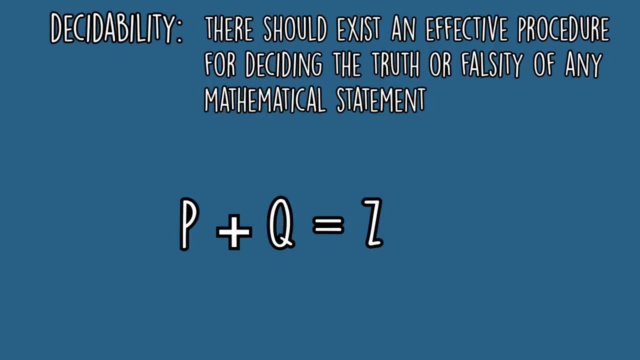 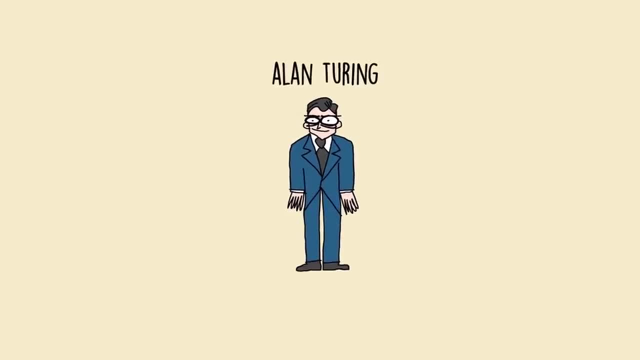 there should be some effective procedure for deciding whether this statement is true within the system. This is where our hero of the story comes in. The hero of the story story comes along, Alan Turing. You may know him from such films as The Imitation Game or the. 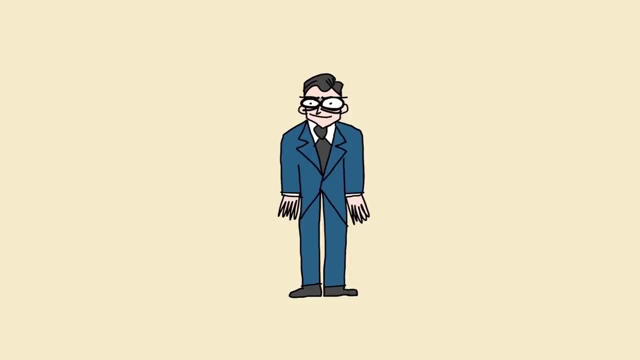 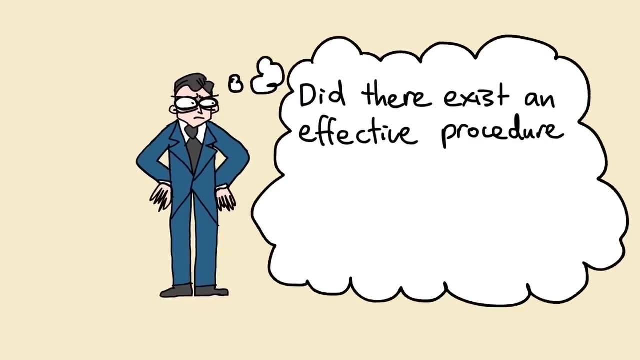 biggest award in computer science, called the Turing Award. At the young age of 22,, Turing got intensely interested in this last question: decidability- Did there exist an effective procedure for deciding the truth or falsity of any mathematical statement? But Turing saw a slight 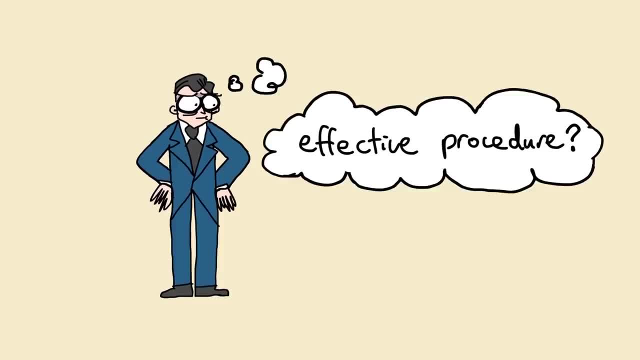 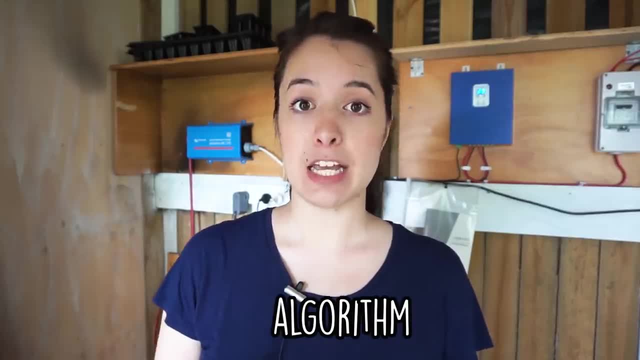 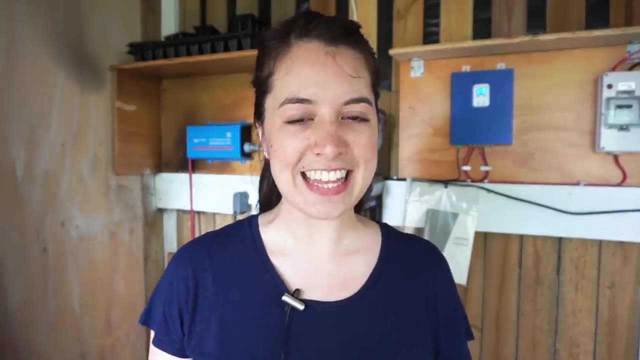 problem with the question: What exactly was an effective procedure? Today, an effective procedure is considered to be an algorithm, some step-by-step set of instructions that you can follow without using any real thought or intuition. But this was back in the 30s and the idea of an algorithm was: 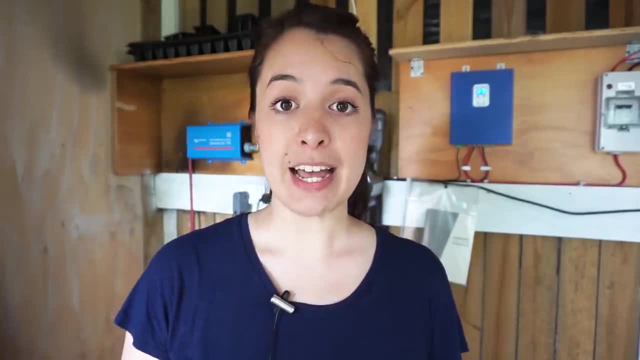 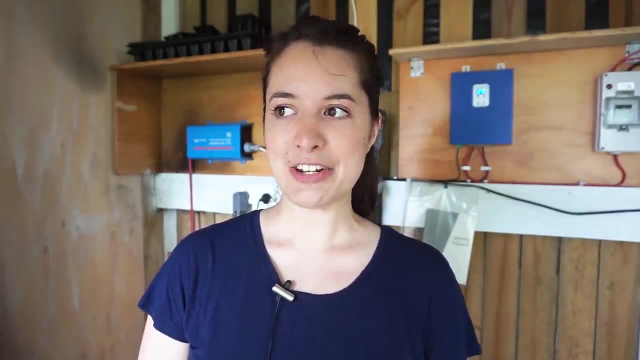 still vague and ill-defined. We're used to the concept now because they're fundamental to how computers work. but computers didn't exist back then, or at least not as we know them today. The word computer referred to people, usually women, who were given a list of instructions. 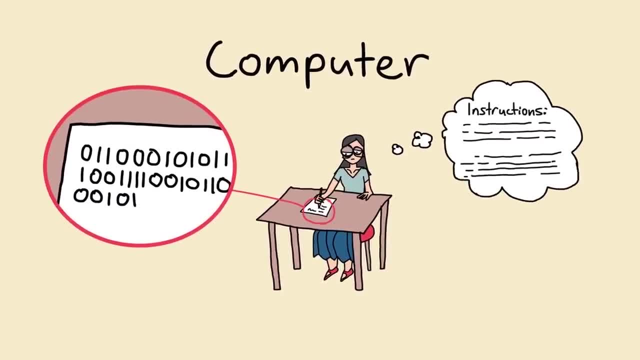 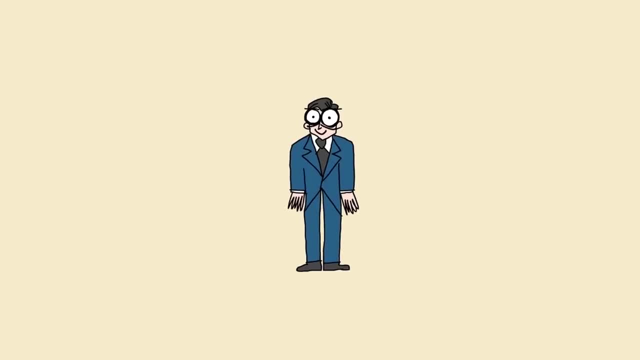 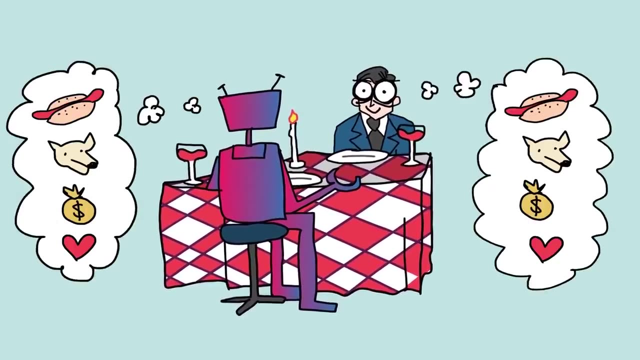 and carried out the procedure. This job required little thought and definitely no mathematical intuition. Throughout his life, Turing was fascinated with the relationship between humans and machines. He's famous for coming up with the idea of the Turing test, a test for determining whether a machine is capable of. 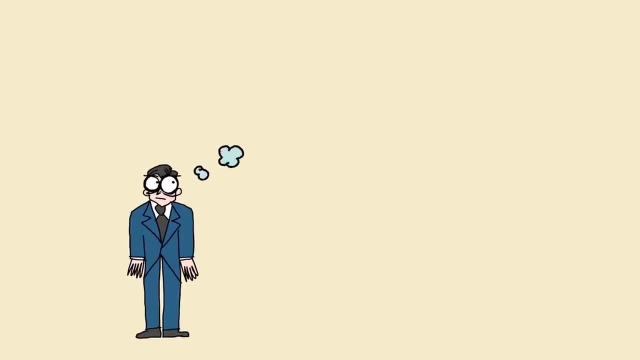 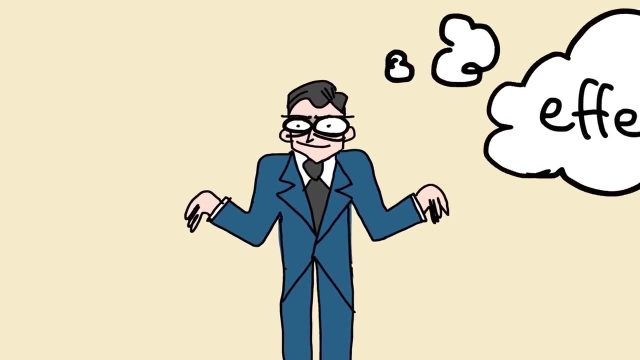 thinking like a human. This was no exception. As the term effective procedure was too vague to do anything rigorous with, he decided to define it himself. He based his definition on a human computer. Turing decided that anything a human computer could do by mindlessly following a list of 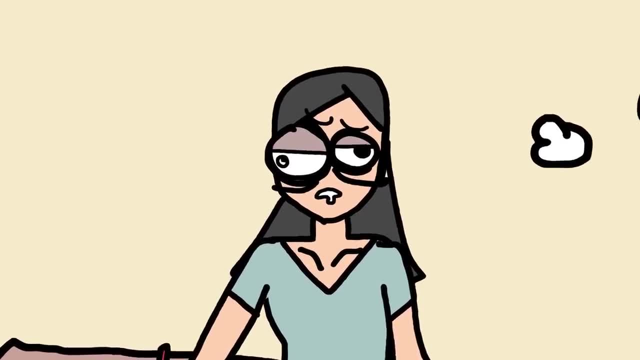 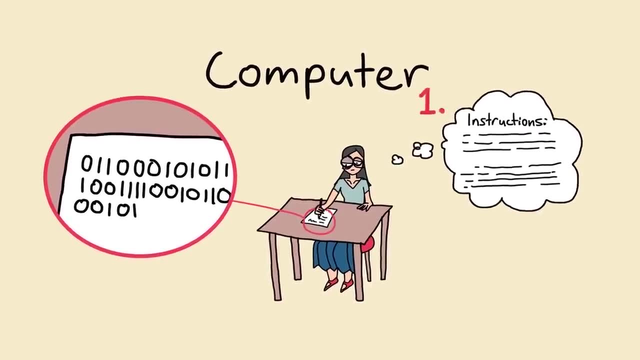 instructions using no genius or insight whatsoever was an effective procedure. He thought about the basic components of what a human computer does when they're computing. One: they read instructions. Two: they read and write symbols on a piece of paper. according to. 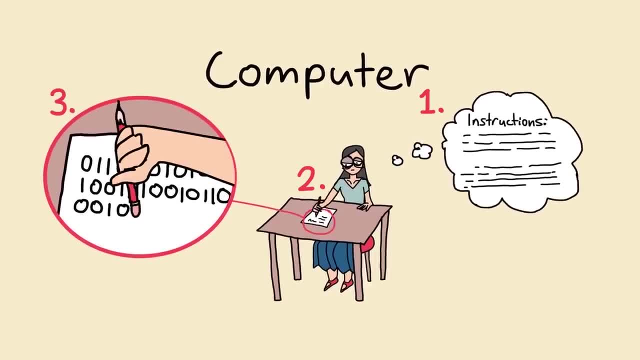 the instructions. Three, they occasionally erase symbols and replace them with new symbols. And four, when they're finished with the computation, they stop. That was about it, And here is where the truly revolutionary part comes in. that would transform the world for years. 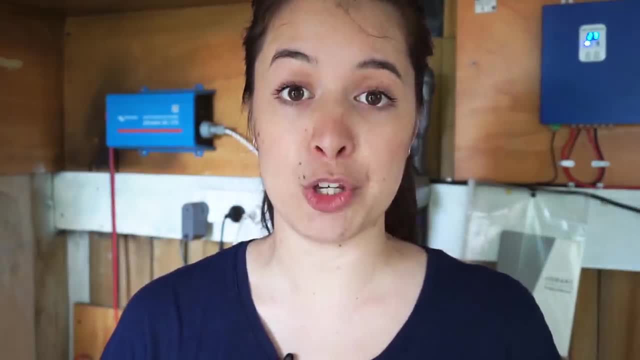 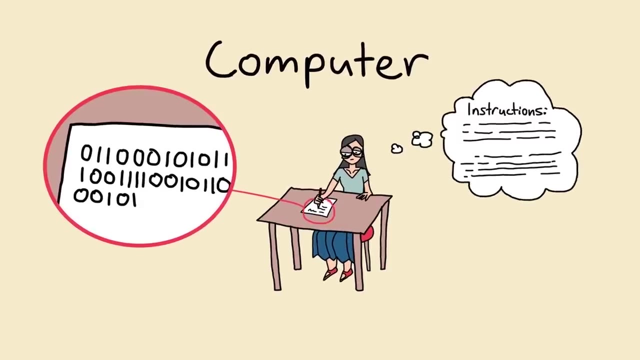 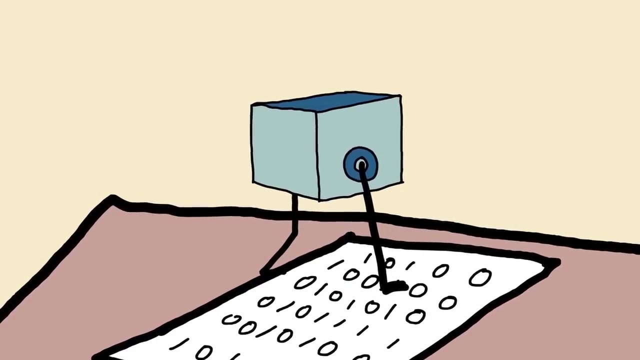 to come. Turing recognized that every step of what a human computer did could be replicated by a very simple theoretical machine. In place of the human could be a scanning head which could read one symbol at a time, erase one symbol at a time and write one symbol at a time: The piece of paper. 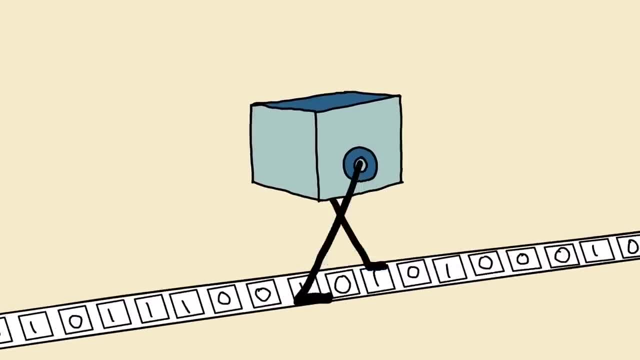 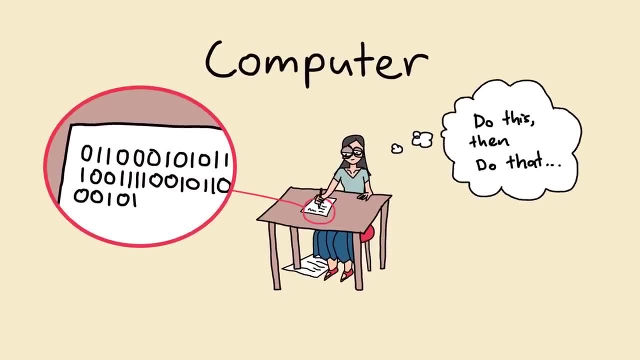 could be replaced by an infinitely long piece of tape which contained one symbol per square. But how does the machine know what to do When a human reads a set of instructions? something is going on in their mind which tells them what to do next. Turing thought of these as 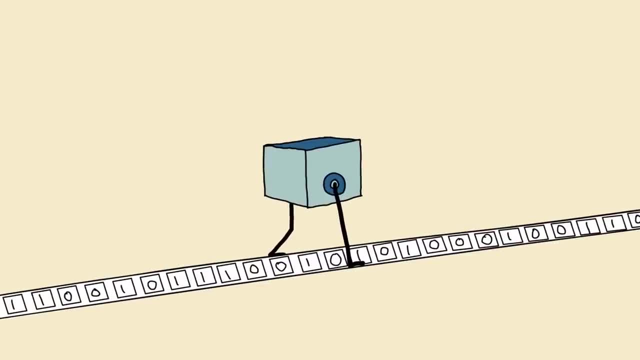 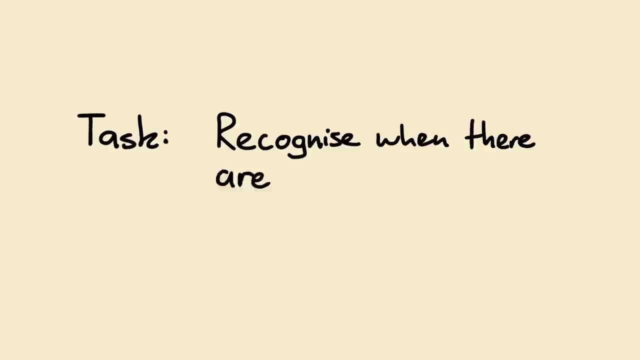 states of mind And so, similarly for his machines, devise the idea of internal states which tell the machine what to do. This idea is best understood using visual diagrams and an example. Say we want the machine to perform the very simple task of recognizing when there are 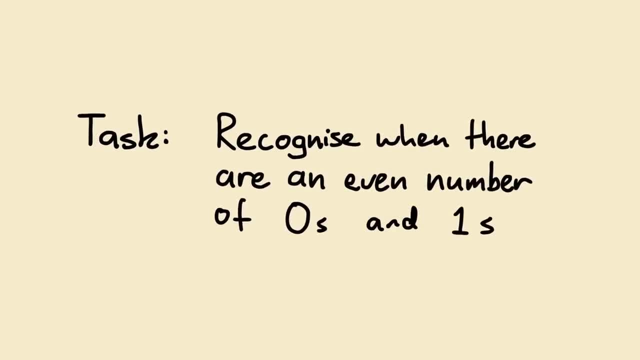 an even number of zeros and ones in the tape, And so we can use the machine to perform the very simple task of recognizing when there are an even number of zeros and ones in the tape. This is easy for a human who has mastered the art of counting, but it's not so straightforward for a machine. 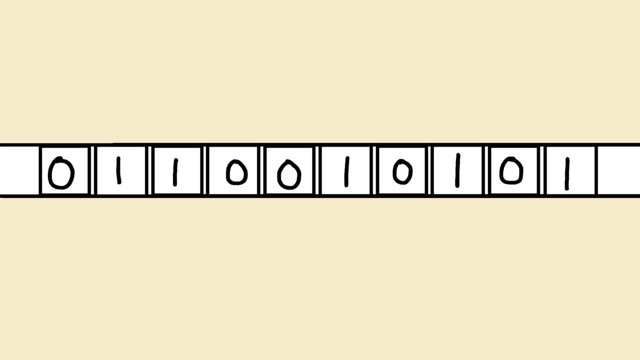 A simple way for our machine to tackle this problem is to pair a zero with a one and then cross off the pair with an x. It keeps doing this until it can't anymore. If it crosses off all the symbols in the tape, we'll know there was an even amount. 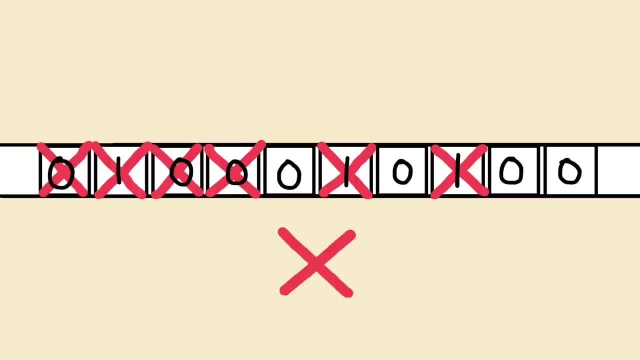 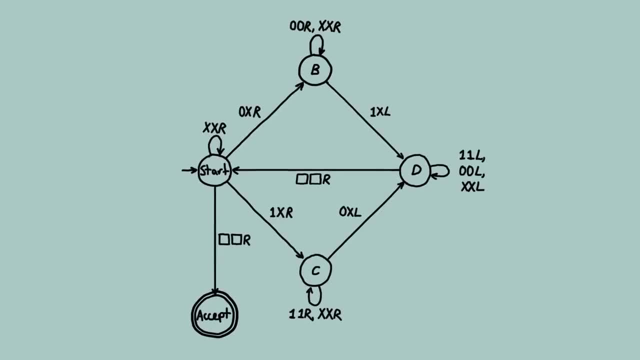 If it doesn't, we'll know that there wasn't. Now, how do we program our machine to carry out this task? Well, we build it with an internal state table that looks like this. I know this looks complicated, but it's not too bad. Let's read it together. 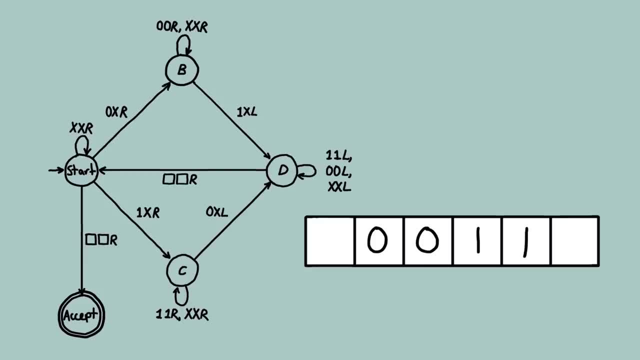 Take this tape with these symbols. We want the machine to tell us whether there is an even number of ones and zeros. The machine starts in the start state. The start state tells the machine: if I find a zero, I will replace it with an X, move to the right and into state B. 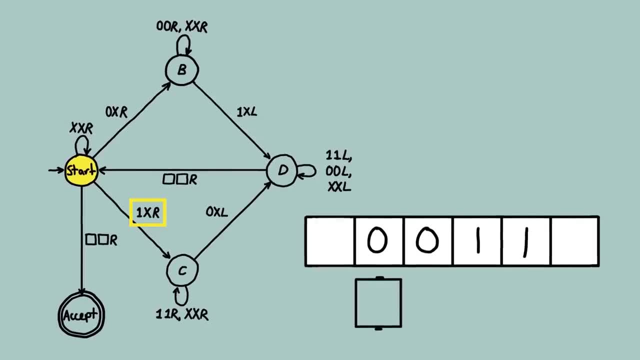 If I find a one, I will replace it with an X, move to the right and into state C. If I find an X, I'll leave it alone and stay in the start state. If I don't find any ones or zeros, and only encounter blank squares, 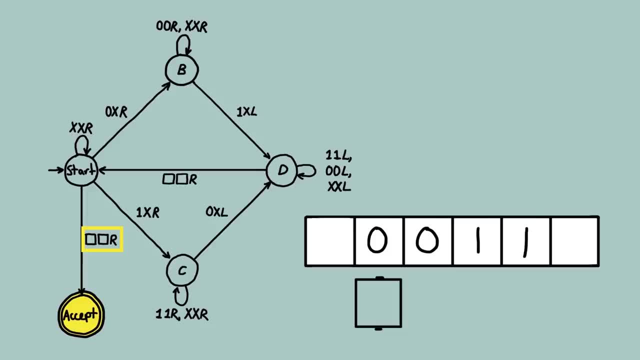 they must have all been paired up. so I move to the accept state. So at the moment our scanning head is in the start state. It reads a zero. replace it with an X. move to the right and into state B. It reads a one. replace it with an X. move one square to the right and into state B. 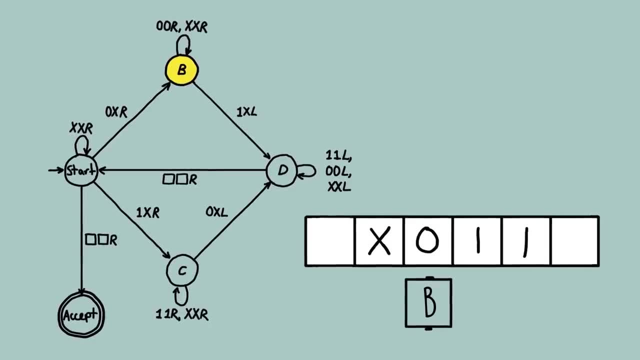 Now the machine has just seen a zero and needs to find a one to pair it with. So state B says: if I see a zero or an X, I'll leave them alone and move right one square and stay in state B. If I see a one, I replace it with an X and move to state D. 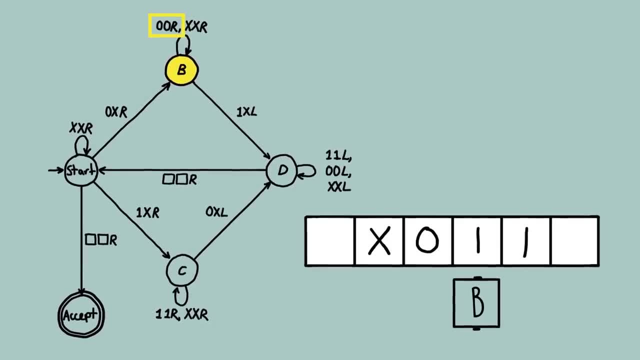 So our scanning head reads a zero, moves one square to the right and stays in state B. Now it reads a one, replaces it with an X and moves one square to the right and stays in state D. Now it reads a one, replaces it with an X and moves one square to the right and stays in state D. 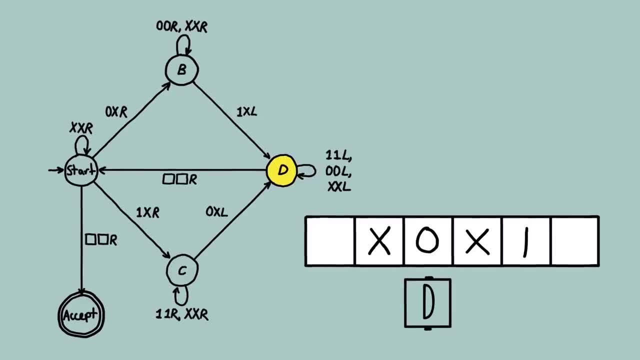 State D is only entered when a zero-one pair has been crossed out by Xs. So the machine needs to reset for the next count. It says. I keep moving the scanning head to the left, ignoring everything. If I see a one, I leave it as a one. 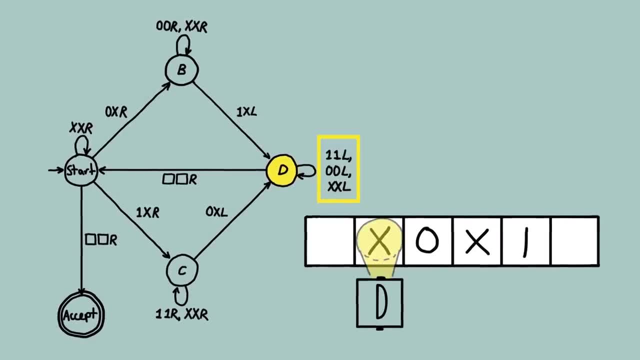 If I see a zero, I leave it as a zero, And if I see an X, I leave it as an X. I keep moving until I reach a blank square, which indicates I've reached the beginning of the list of symbols. I then move one square to the left and into state D. 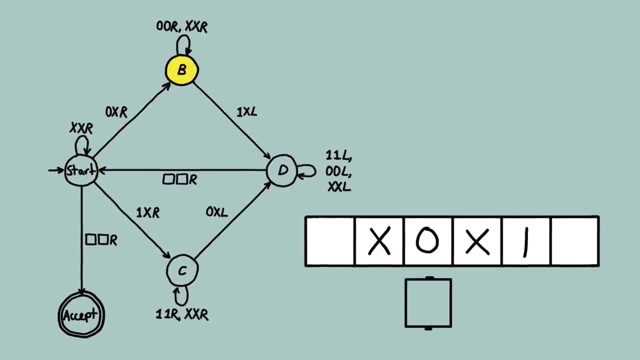 I move one square to the right and go back to the start state to repeat the whole process. After another round of this, the machine only encounters Xs, so keeps moving right and remains in the start state. When it reaches a blank, it moves into the accept state. 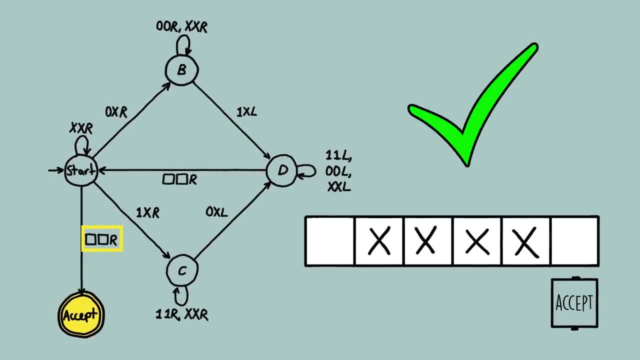 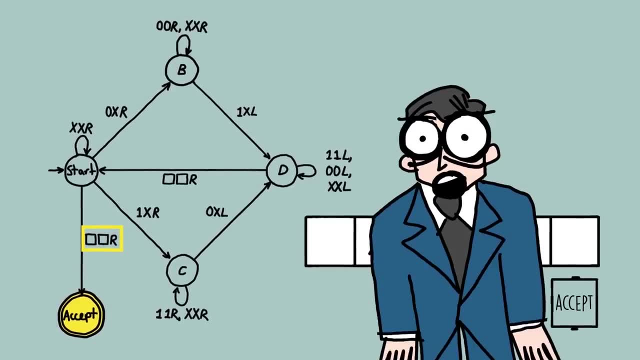 and we know that this list of symbols does have an even number of ones and zeros. So that's how one of these machines would work. But here Turing had another incredible insight. See, at the moment you would need to build different machines to do different tasks. 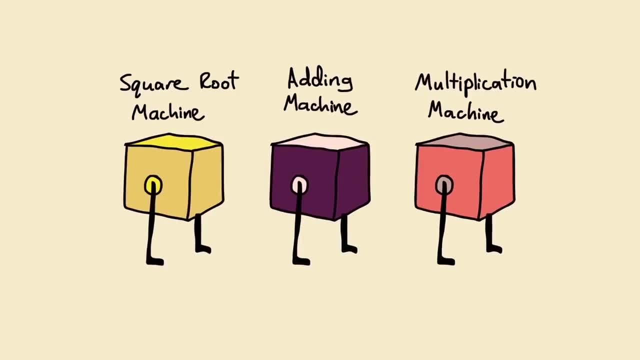 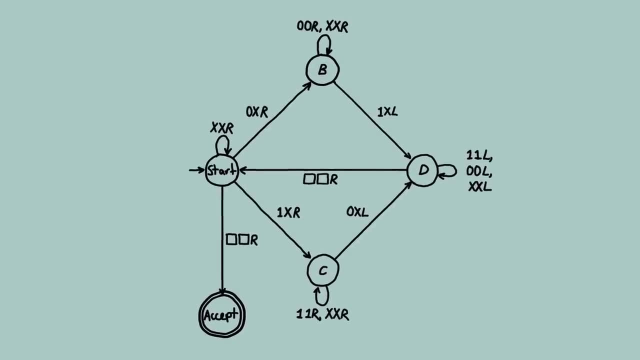 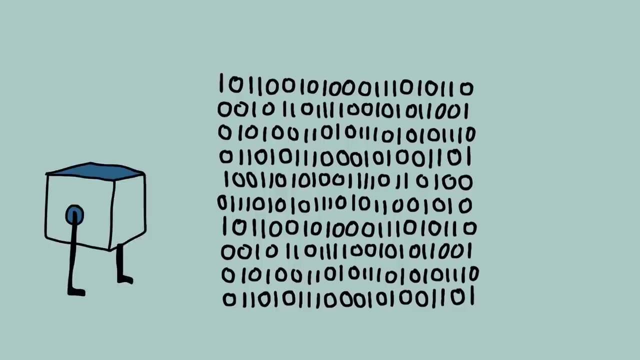 A machine to calculate square roots would need to be built with a different internal state table than a machine to do addition. But Turing realized that any internal state table could be encoded into a list of ones and zeros. In this way we could feed the instructions as well as the problem into a new machine. 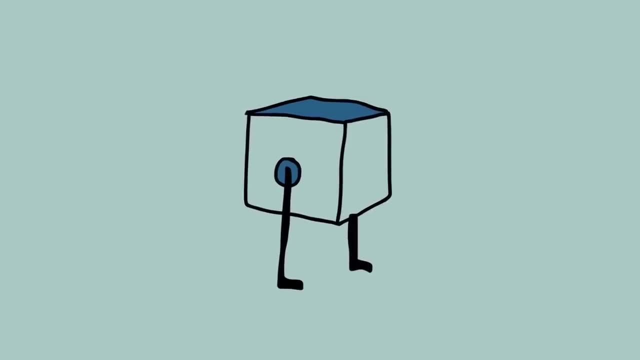 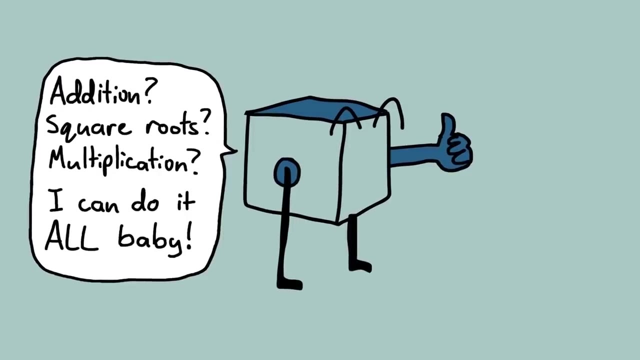 and that machine could perform that set of instructions. Today we know this as a programmable computer. We have computers which we can program to do different things after they've been built. That idea originated right here in Turing's paper. He dreamed up a theoretical machine that could perform the same task as any other of his machines. 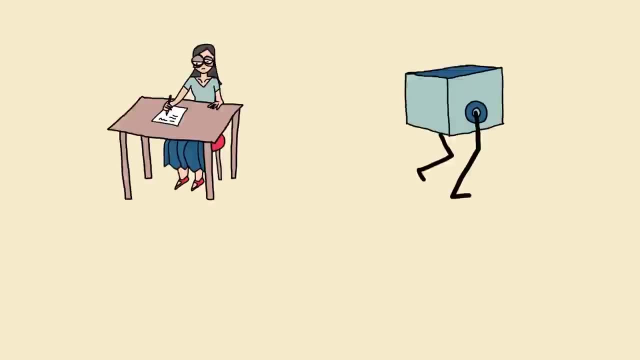 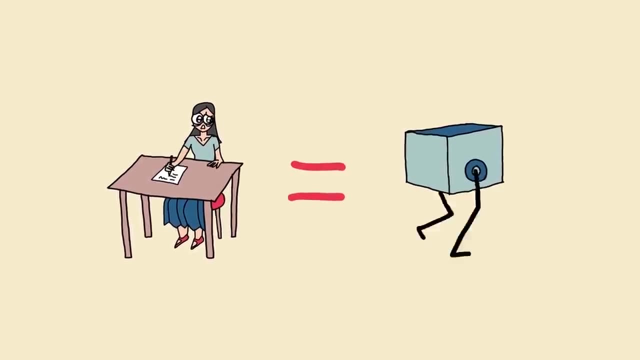 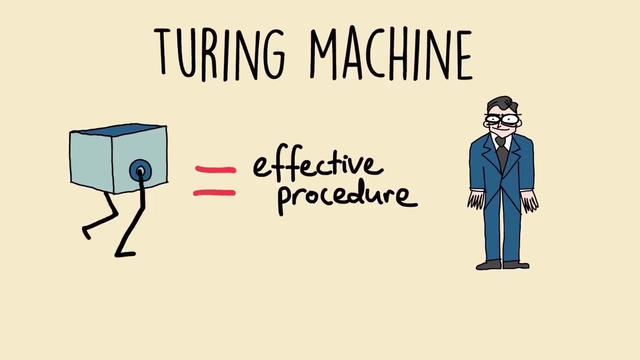 and that was pretty freaking incredible. Even though this theoretical machine is incredibly simple, it can, in principle, do everything that a human computer can do. This abstract machine, now called a Turing machine, was Turing's definition of an effective procedure. An effective procedure was anything that could be computed. 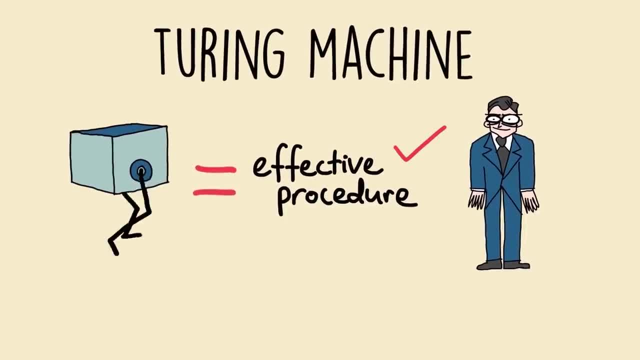 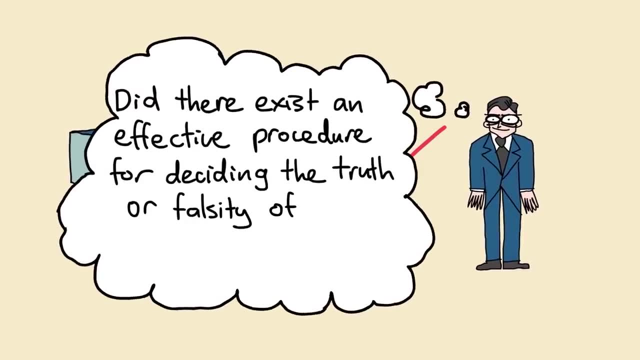 by a Turing machine in a finite amount of time. So with that out of the way he could go on to answer Hilbert's question, Did there exist an effective procedure for deciding the truth or falsity of any mathematical statement Or as framed by Turing? 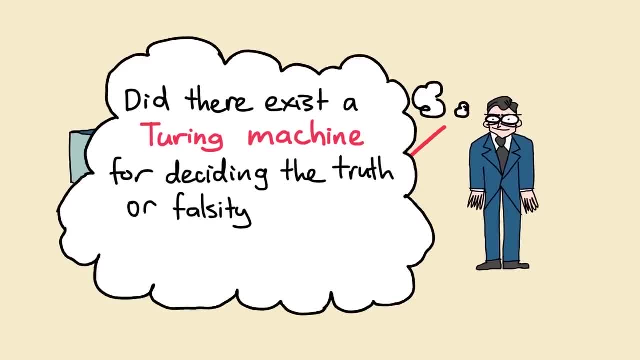 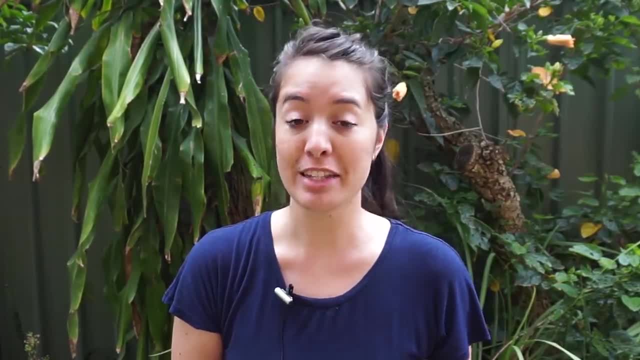 did there exist a Turing machine for deciding the truth or falsity of any mathematical statement? The way that Turing answered this is beyond the scope of this video. I did make an entire separate video about it, called The Halting Problem, which you can check out after this. 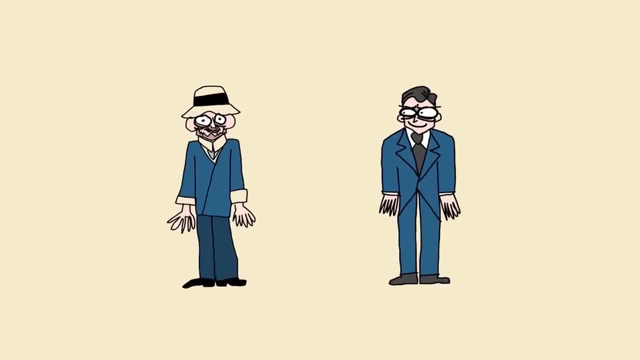 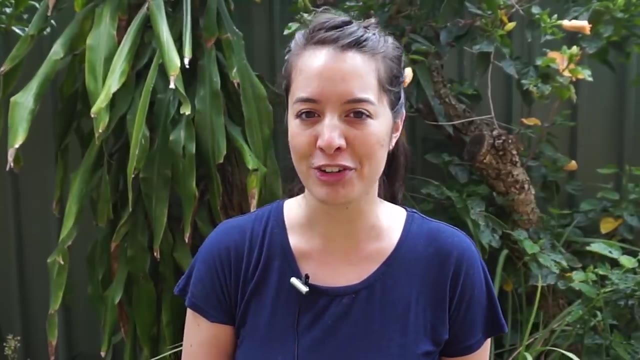 But I will tell you that Hilbert's program ended in complete failure, and Turing contributed to it by proving that there was not an effective procedure for deciding whether any mathematical statement was true or false. This alone is an amazing achievement, but Turing's little machines took on a life of their own. 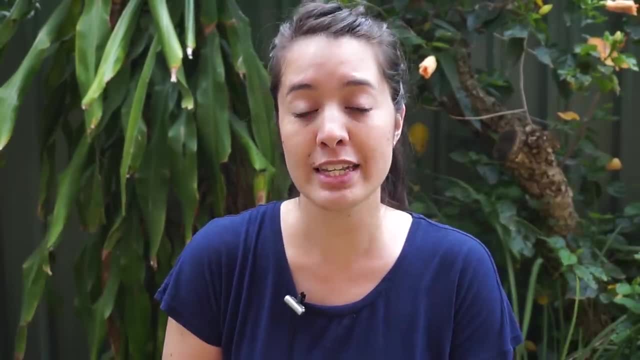 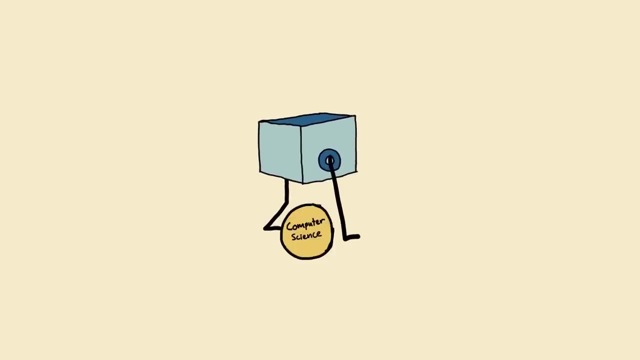 By making a definition of computation that was rigorous, people were able to study the nature of computation and its limitations like never before. This birthed the entire field of computer science, which is the study of what computers can and can't do. the complexity of algorithms. 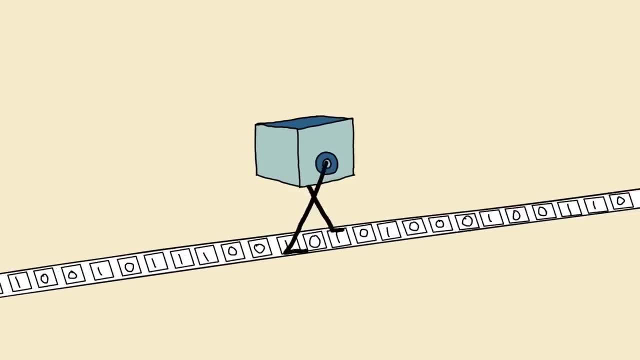 and the overall nature of computation. Furthermore, by coming up with an intuitive, easy-to-understand model, people were able to turn the abstract and vague notion of computation into a physical machine that could replicate the process. Turing machines are the blueprint of the modern-day computer. 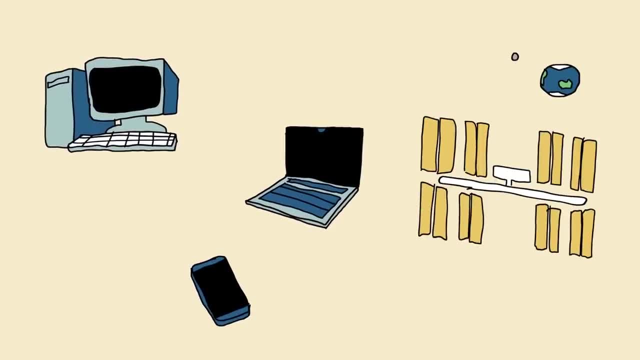 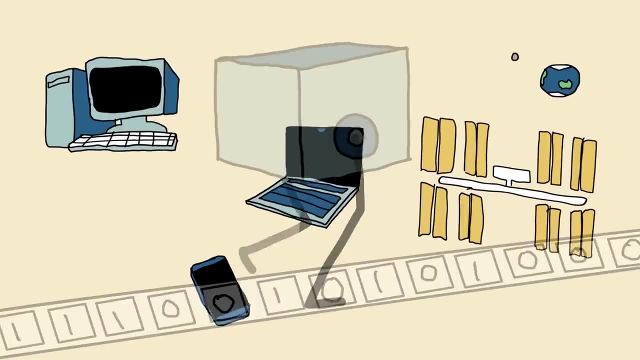 Anything from your desktop to your smartphone, to the computers on the International Space Station, are based on Turing's model. Anything that any of these machines can do can, in principle, be done. It might just take a bit longer. Now, it's worth noting that other models of computation do exist. 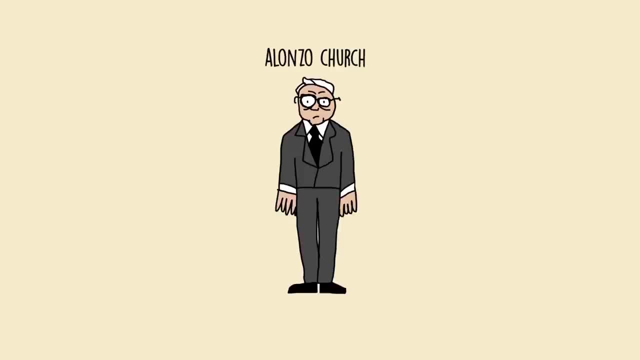 Alonzo Church, who would later become Turing's doctoral advisor, actually came up with his own model just weeks before Turing called the Lambda Calculus. Turing found out about this just before publishing his own paper and wrote a quick appendix which showed that Church's Lambda Calculus 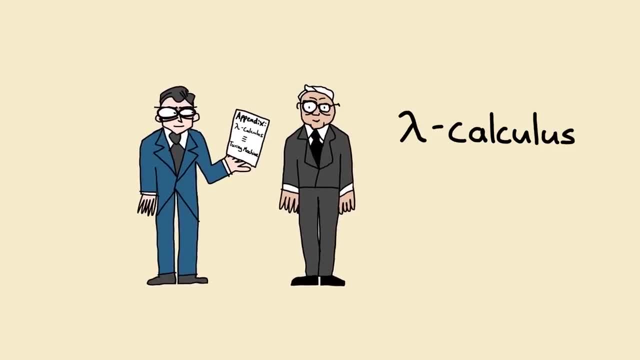 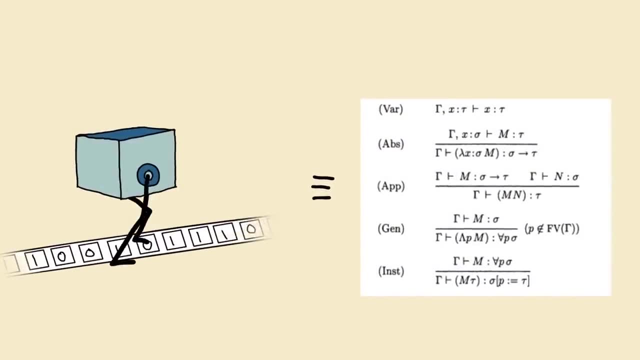 and his own model were in fact, equivalent, meaning that anything that can be computed by the Lambda Calculus can also be computed by a Turing model. So if you want to learn more about the Lambda Calculus, you might want to check out the video on Turing's Lambda Calculus. 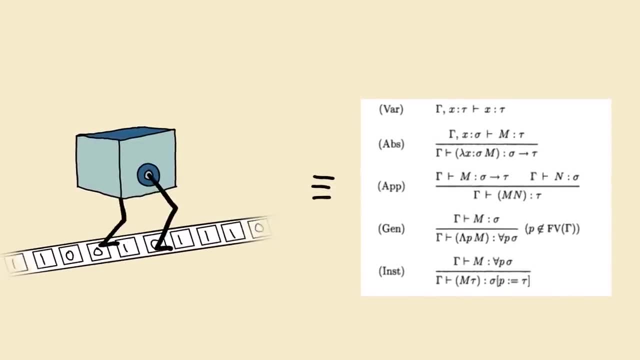 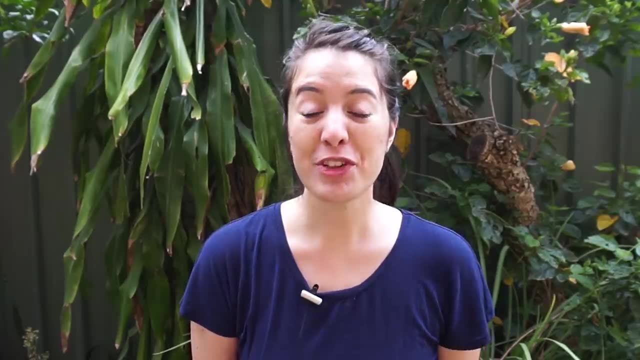 Turing's Lambda Calculus is a model of computation that can be computed by a Turing machine and vice versa. However, because of their concreteness, simplicity and precision, Turing machines were the model that caught on and captivated the imaginations of the mathematics community. 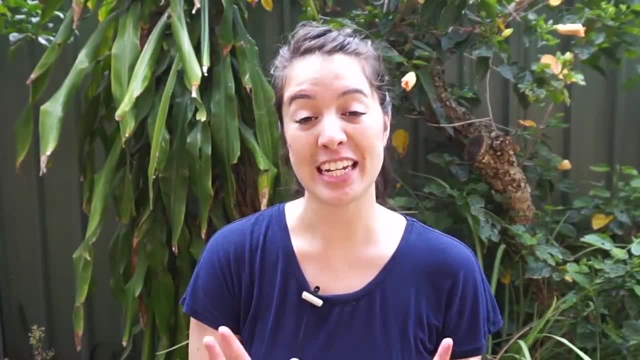 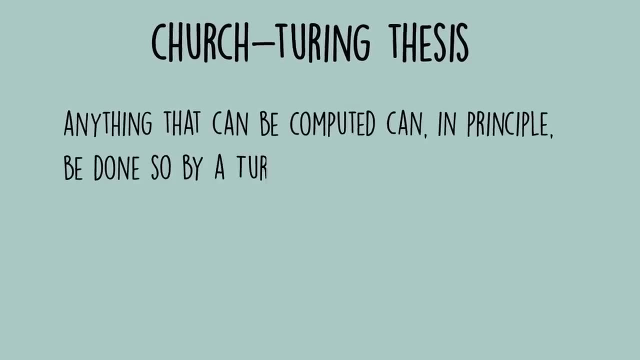 Even though they were conceived nearly 90 years ago, there is currently no working model of computation more powerful than Turing's. This is embodied in the Church-Turing thesis, which states that anything that can be computed but can't compute it, it's not computable. That's not to say that this might not someday change. There's a growing field of study called hypercomputation, which studies theoretical models of computation more powerful than Turing machines. The trouble is making them physically realisable. Another model of computation that's been getting a lot of hype recently: 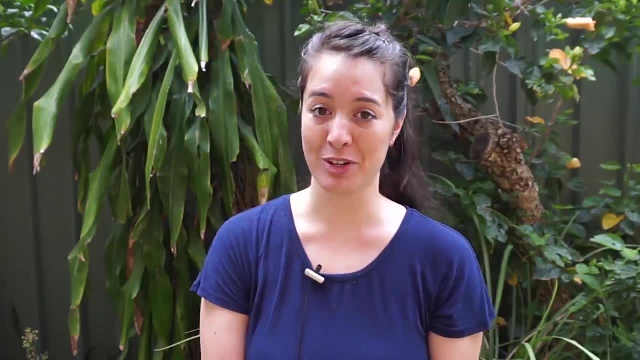 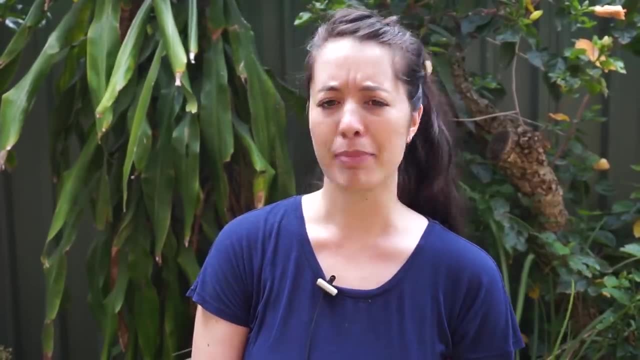 are quantum computers which, if they work, will definitely bring something new to the table. But so far Turing's simple model, which he dreamed up at age 22,- kind of as a byproduct to answer a totally different question- is still the most widespread model of computation to date. 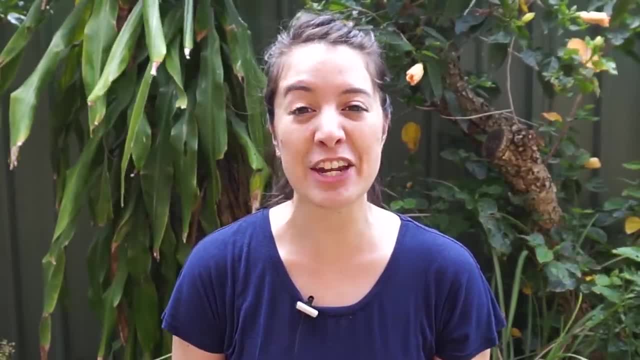 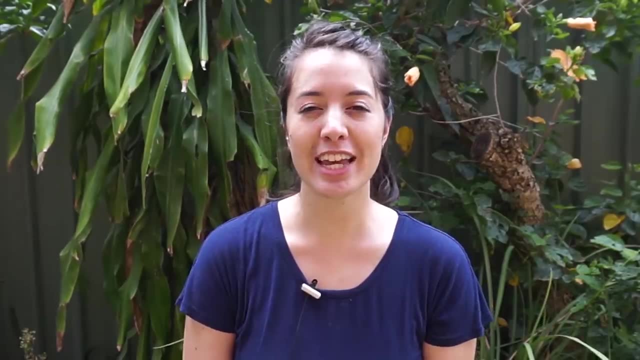 This video was an origin story about one of the most fascinating and relevant fields of study, But there is so much more to computers and algorithm that's worth exploring. If you'd like to get a real handle on the fundamentals of computer science, hearing about it in a video probably isn't enough. 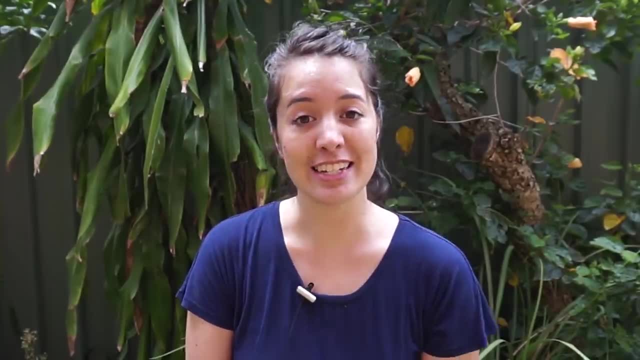 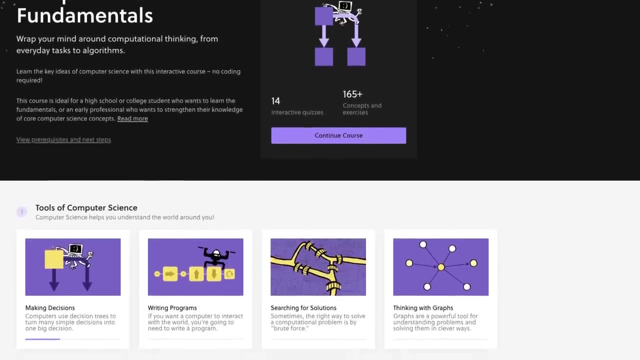 But there is good news: You can learn about it, The same way I did Through interactive courses on Brilliant. In this computer science fundamentals course, you can learn how to write programs, search for solutions using the computational method of brute force and make your own algorithms.